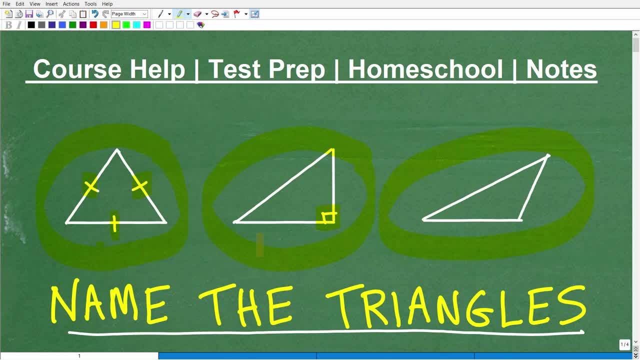 six I'm going to go over and if you know the names of these three, go ahead and put those in the comment section and we'll see how well you do here in just a second. but first let me quickly introduce myself. my name is John. I'm the founder of Tablet Class Math. I'm also a middle and high 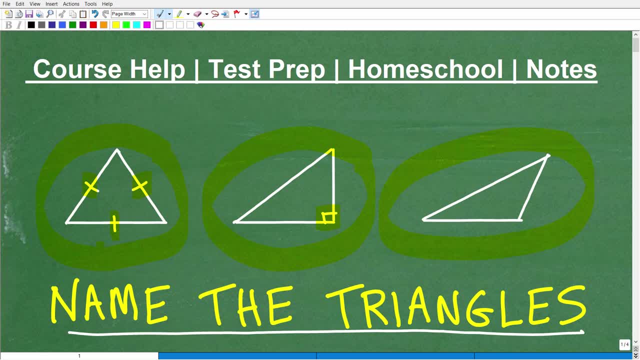 school math teacher. I'm going to leave a link to my math help program in the description of this video. but if you are frustrated in math right now, maybe you don't feel like you're getting enough math instruction, or maybe you're not connecting with your teacher's teaching style. whatever the 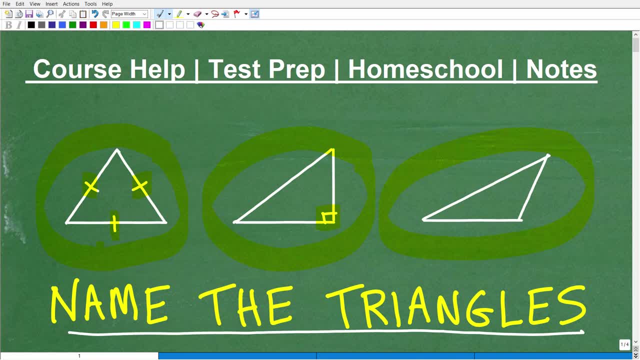 case is, I've been teaching math for decades. I really try to strive on teaching math in just bite-sized pieces so anyone can understand, and I really focus on teaching math in a clear and understandable way. so if you're at the middle school, high school, even college level in terms, 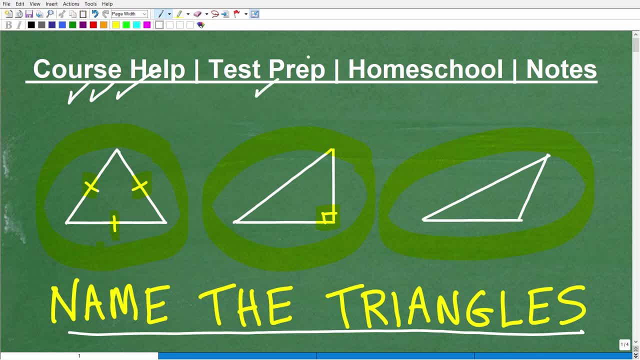 of mathematics. I can help you succeed now if you're preparing for any test that has a math section on it. so I'm talking about things like the GED, SAT, ACT, GRE, GMAT, ASVAB, ACCUPLACER, ALEKS exam, maybe a teacher certification exam. you get the idea. I can help you prepare and pass those exams. 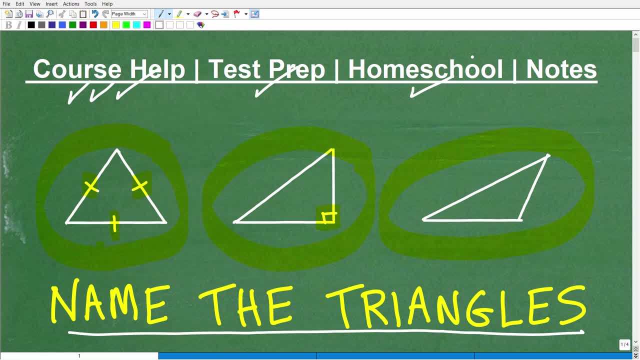 if you homeschool have a teacher certification, you get the idea I can help you prepare and pass those exams. if you homeschool have a teacher certification exam, you get the idea I can help you prepare and pass those exams. if you homeschool have a fantastic homeschool math program, And if you need some math notes, don't panic, I'm going. 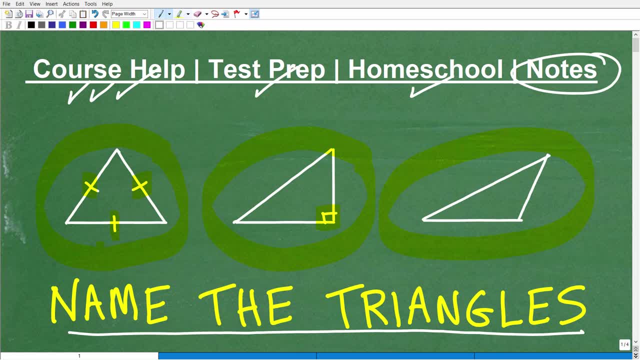 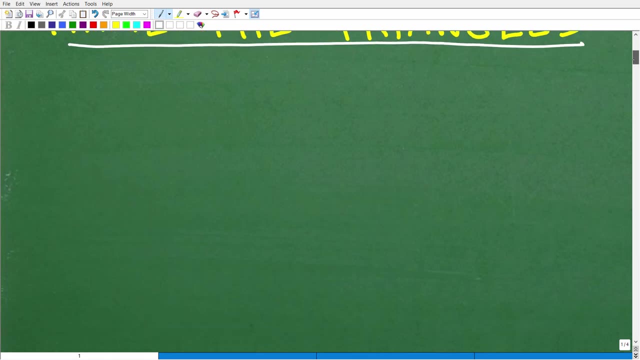 to leave links to my math notes in the description of this video, But if you want great grades in mathematics, you must absolutely take great math notes. Okay, so we're going to cover these three triangles and three more, So let's go ahead and get to it. I'm just going to show you all six of 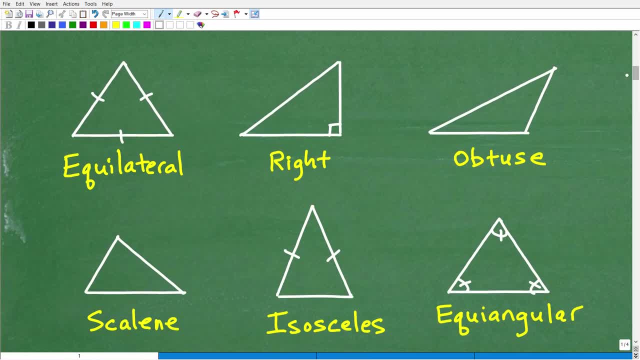 these triangles and then we'll kind of get into how we define how the name matches the shape. All right, so this first triangle, okay, and this is no particular order, but these are the first three that we looked at. So the answer for this one would be an equilateral triangle. So this is. 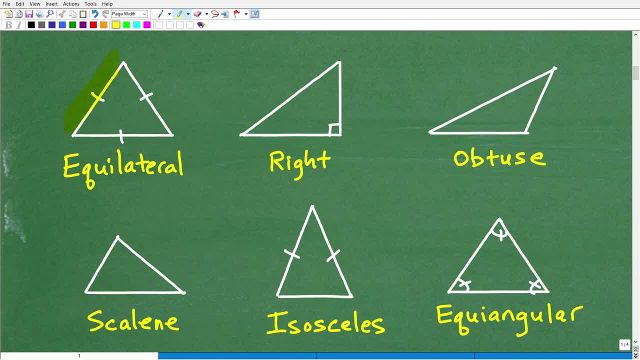 an equilateral triangle, which means that all the sides here are equal. Okay, so this little notch right there on the side, this is indicating that this length is congruent to this length and both of those lengths is congruent to this length, ie they have the same sides. 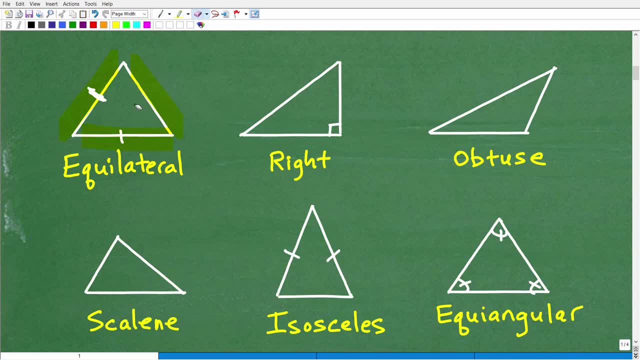 Now, if you look at this triangle, you'll see that the sides are the same. So this is the same length and both of those lengths are congruent to this length, ie they have the same sides. Now, another way you could see an equilateral triangle. you may not have that notation. You might be. 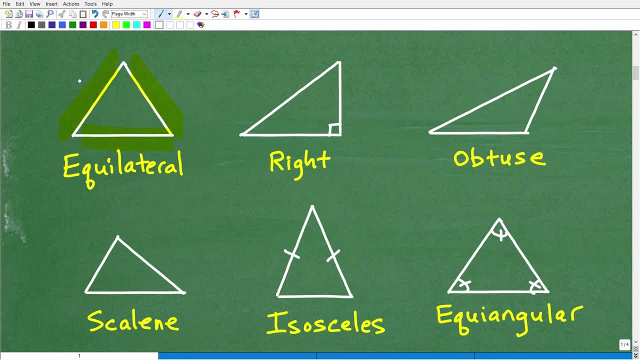 actually given, let's say, the actual sides. You might get like three, three and three, And here you say, oh okay, all the sides are equal, so equilaterals. That's our first one there. Now, 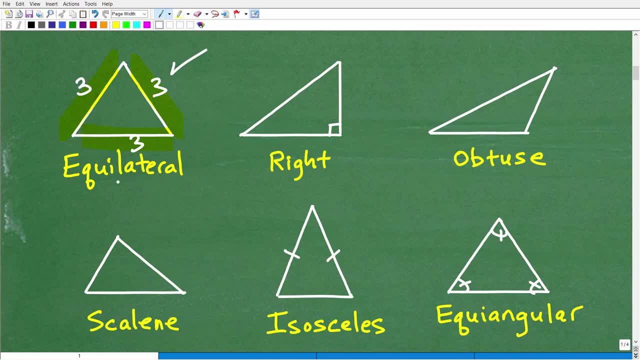 the equilateral triangle has something in common with this other one that we're going to be looking at here. our last triangle, That's the equal angular triangle, But what we're going to do is we'll talk about that in a second, So let's move on to our next triangle. That is a right. 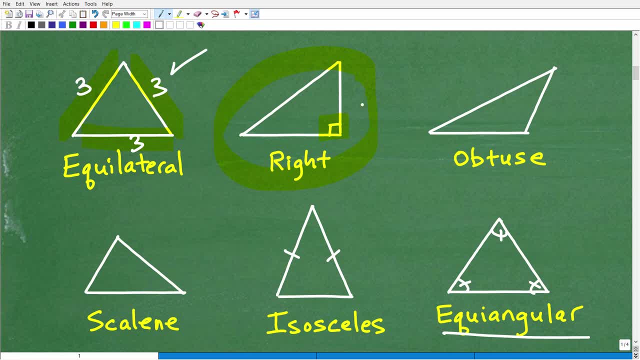 triangle, okay, Very, very important triangle in geometry and mathematics, and it's indicated by this little box down there. And that box- okay, that little tiny box in the corner, is saying that this is a 90-degree angle. Now one thing you need to know: that in all triangles, the sum 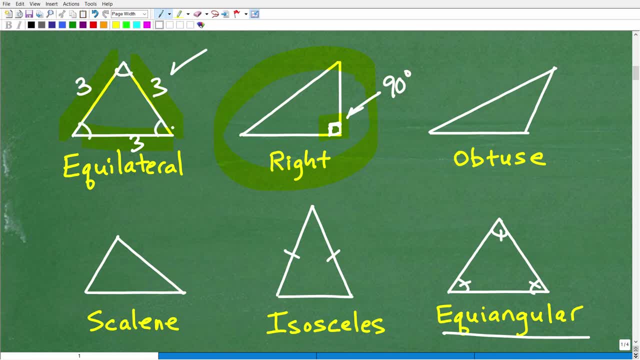 of the angles. in other words, this angle plus this angle plus this angle, any triangle you have- all these triangles that we're looking at here- always adds up to 180 degrees, But in a right triangle, one of those angles is 90 degrees. 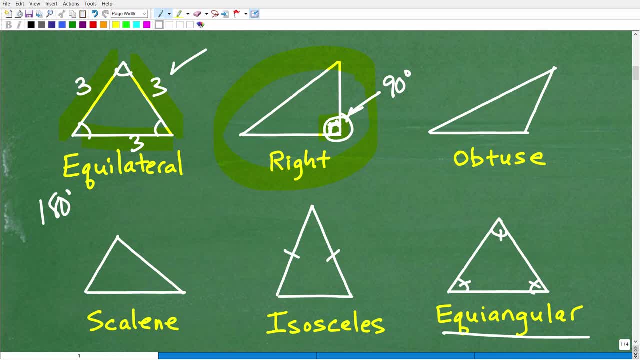 and it's indicated by this little mark right there, that little box. okay, So right, triangle, extremely important triangle in geometry. Now, for some of you out there, you might be familiar with the Pythagorean theorem: a squared plus b squared is equal to c squared, That relationship. 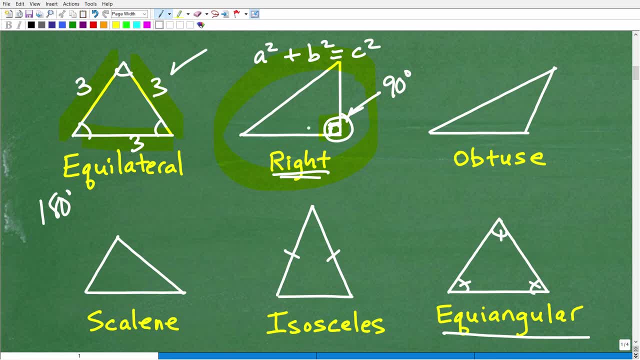 only applies to right triangles, not these other type of triangles. There is a another type of theorem, called the law of sines and cosines, that we can apply. That's a little bit more advanced mathematics. but this right here only applies to right triangles. That's why 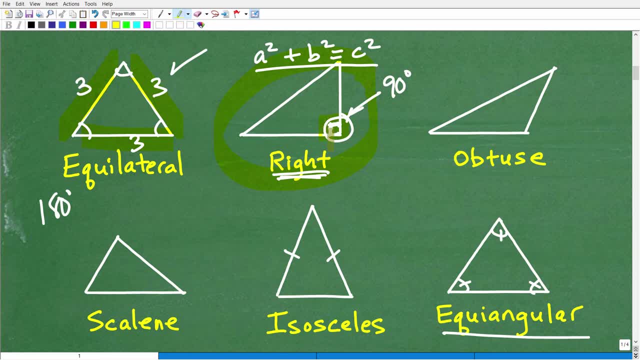 it's important to know these names or be able to recognize what type of triangle based upon the notation. All right, let's go ahead and talk about this next triangle. This is an obtuse triangle. okay, That's the name of it, And the reason why it's obtuse is one of the angles is greater than. 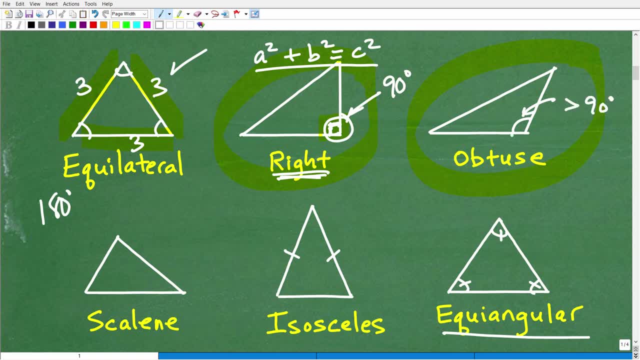 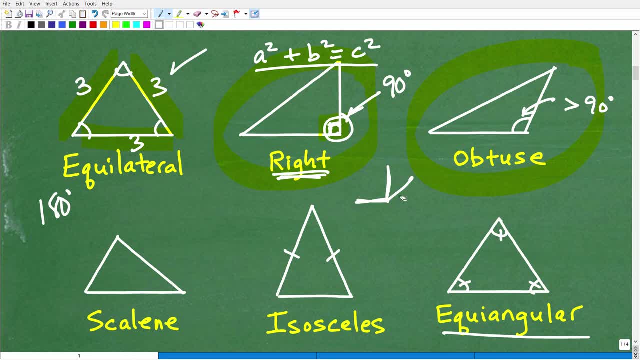 it's like a perfect corner on a square. So if you got a triangle that has an angle bigger than that, like this right here, that's obtuse. Now there is another name that kind of goes the opposite with obtuse, which would be acute. okay, An acute triangle, Now it's not on here. 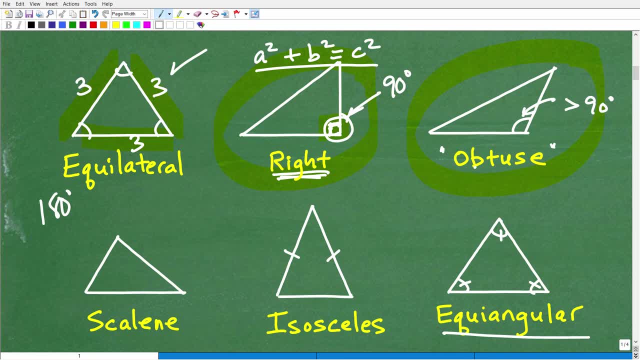 but it's something that you want to know anyways- is a triangle where all the angles are less than 90 degrees, So maybe like an equilateral- this one that we're going to be talking about here in a second, But obtuse. again, one of the angles is greater than 90 degrees. 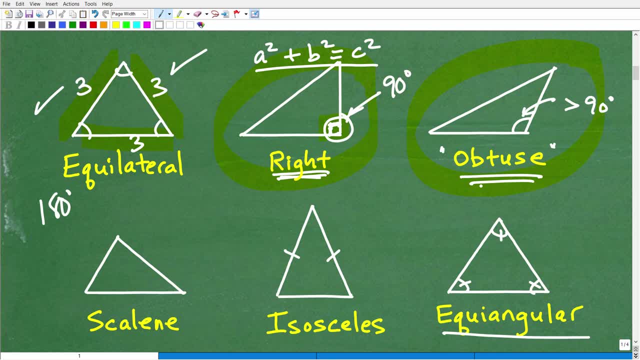 It's kind of funny how we use some of these names too. like you know, there's an adjective you could say, well, that person's obtuse, which means that maybe they're kind of, you know, dull, or maybe they're not. you know, you know someone's saying they're not too bright. 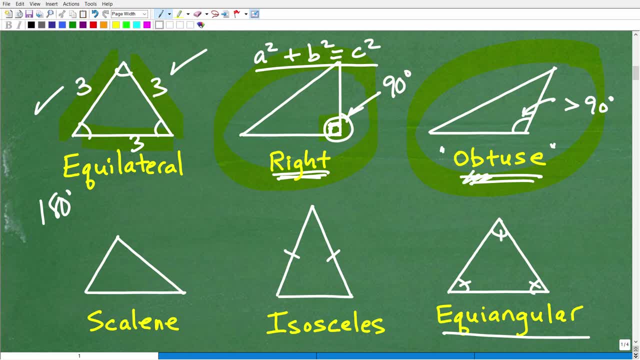 whatever the case is, you'll hear this word used in other ways- obtuse- just as you use the word acute. okay, Oh, I have acute pain, sharp pain. Well, the opposite of sharp is dull, right, And that's what obtuse is, Okay. so let's move on to our 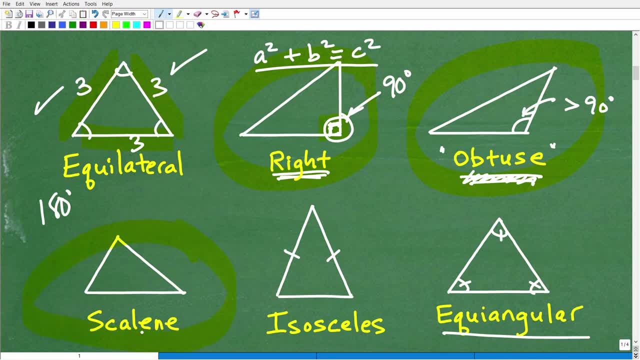 next triangle, That is the scalene. Now, what do you think makes the scalene? I'm trying to kind of draw this in such a way where you kind of really kind of see what's going on- But what do you think makes the scalene triangle a scalene triangle? Okay, well, if you look at it here, 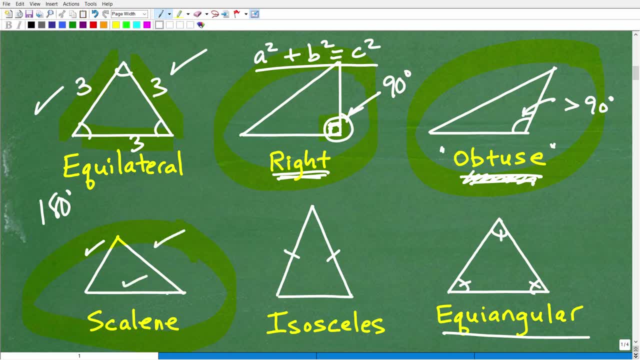 hopefully you're saying: well, it doesn't look like. well, three sides are different lengths. Well, and that's that's what you said. That's exactly correct. So a scalene triangle is where all three sides are different lengths. Okay now 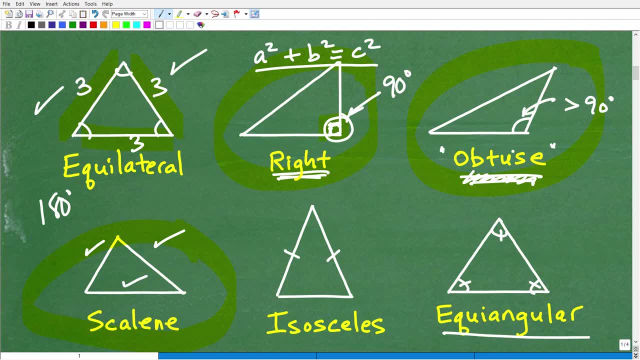 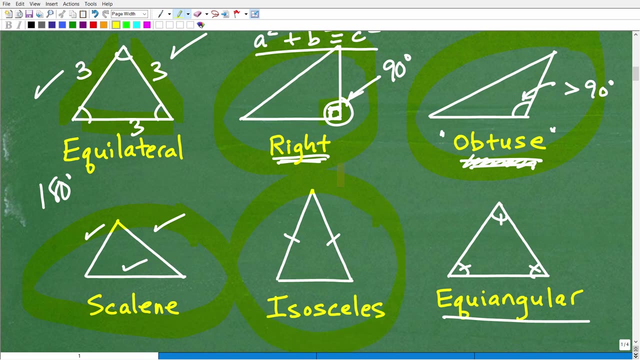 even though you might have an obtuse triangle and the sides are different lengths, it's more appropriate to call, like an acute triangle with different lengths, scalene. okay, scalene triangle, All right, let's move on to our last two, And our next one here is going to be the isosceles. 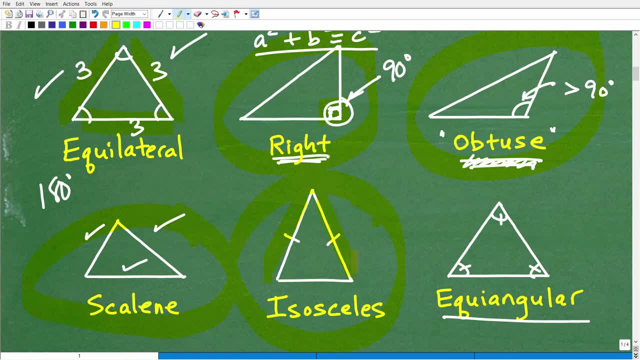 triangle. Okay, so an isosceles triangle is where two sides, not three sides, only two sides- are the same length, And so this would be like the base and this would be the sides right here. Now, interesting enough is on a isosceles. 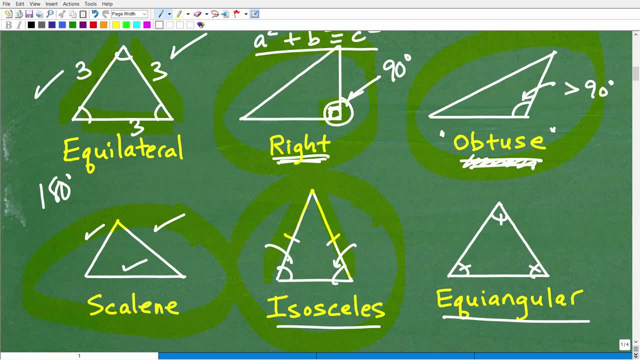 triangle, the base angles right here are congruent. So when you're studying triangles in more detail, we can study different things about isosceles triangles, right triangles, equilateral triangles, et cetera. So again, you know you need to be able to put a 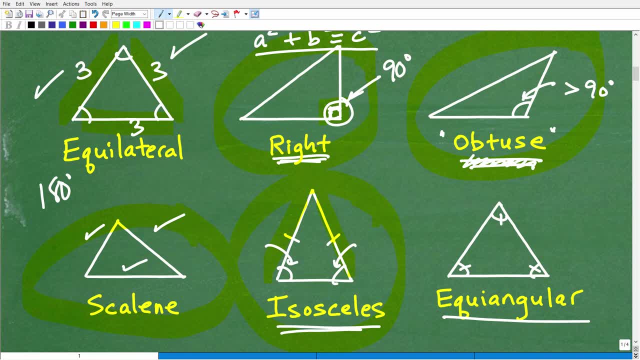 name on whatever particular type of triangle that we're looking at. So isosceles triangle, two sides are congruent, All right, and this leads us to our last triangle, and that is the equal angular triangle, and all three angles are equal. Now let's just do some algebra here. 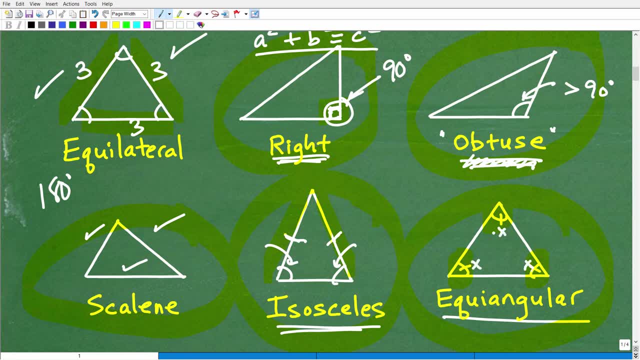 And so, if this is x and this is x and this is x, and I know that x plus x plus x is equal to 180 degrees, what is the angle of an equal? what is the actual angle measure of these angles? Well, this would be what: x plus x plus x. 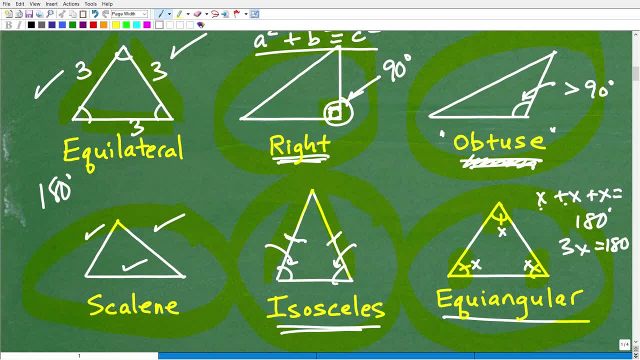 3x is equal to 180.. I divide both sides of the equation by three, so x is equal to 60 degrees. So an equal angular triangle. the angles are 60,, 60,, 60, and over here for equilateral happens to. 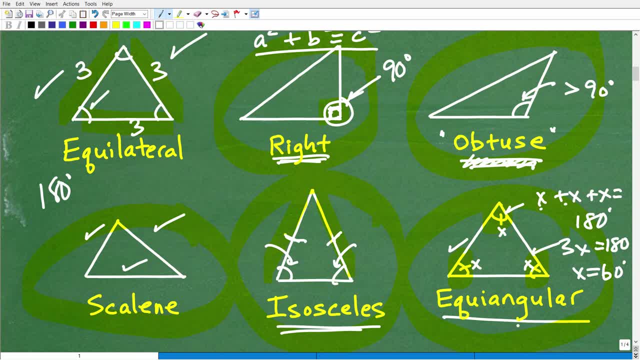 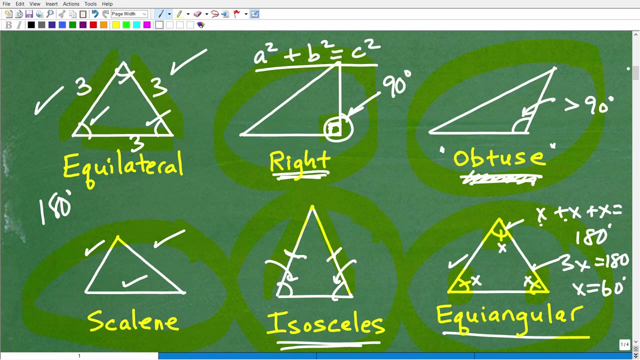 be has the same property as equal angular, So they are both basically the same triangle. Okay, so you have same length and same angles, Okay, so this is basically. the whole point of this video was just basically to get you to know these names. Okay, may not seem important, but it definitely is. 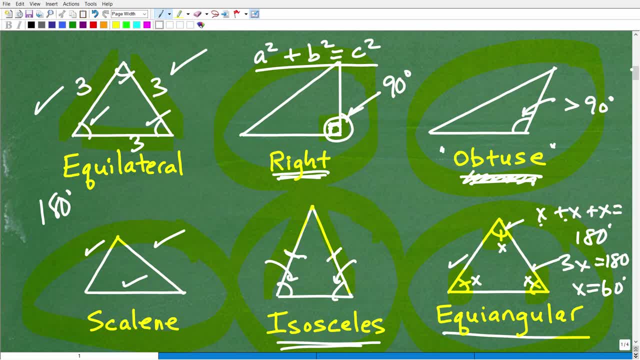 important because you know when we talk in geometry we're talking about particular shapes and figures. we go, they go by particular names And I can almost guarantee you if you're going to be taking any sort of test. a very common type of question, even on standardized tests, is name. 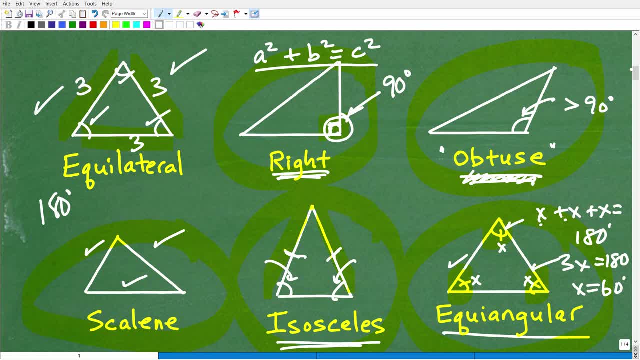 the triangle. Okay, like which is the isosceles triangle? And or they might show you an isosceles triangle and then you'll have to know something about an isosceles triangle. But if you show, if they show you a, 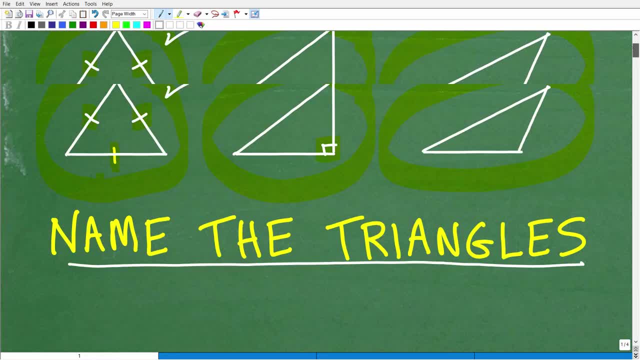 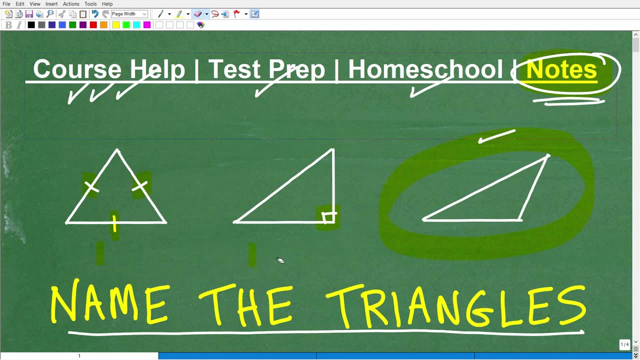 triangle and you don't even know it's an isosceles triangle. well then, you're going to be in trouble, But hopefully this was a. you know you didn't find this difficult. I don't think this is hard, But if you didn't know this, well then hopefully now you do And if this video helps.